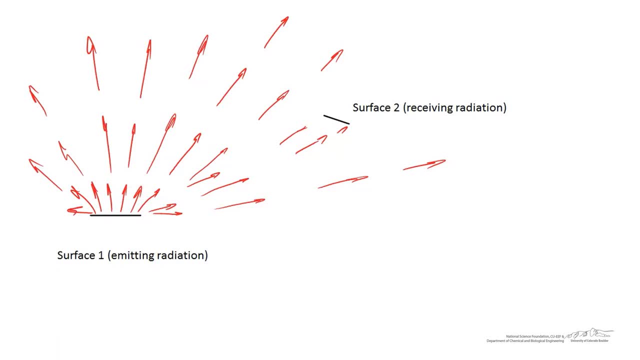 of them for the time being, because there's a couple of things that are worth considering. When we think about, or considering in terms of how much radiation is coming out of surface two, how much radiation is being received by surface two, one thing to consider is the 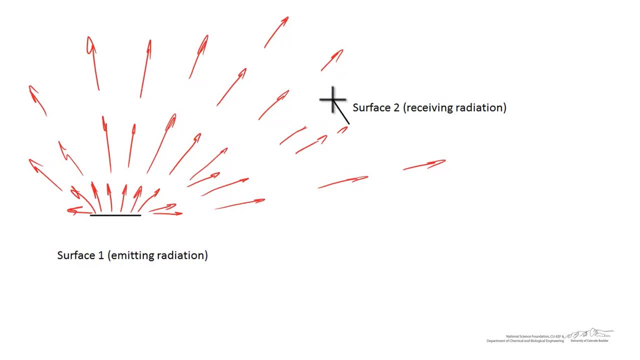 angle of surface two relative to surface one. So if I arranged surface two like this, you can imagine if the angle, if that angle is its unit, normal, if it points directly at surface one or it's completely perpendicular to the radiation impinging on it, it receives. 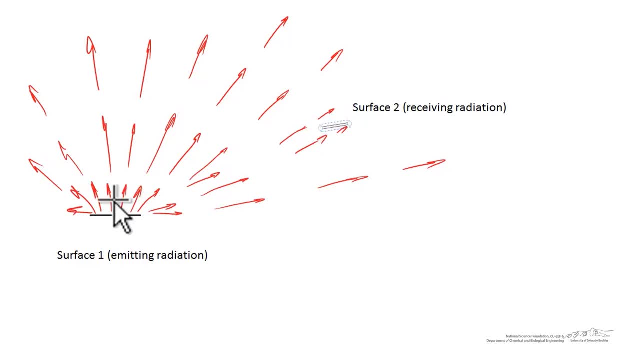 a lot more radiation than if it was at an angle like this. So this angle, most of the radiation just goes by it, It's not received. And in this limit, this angle, there is a no radiation being received whatsoever, Everything just passes by it. assuming this surface. 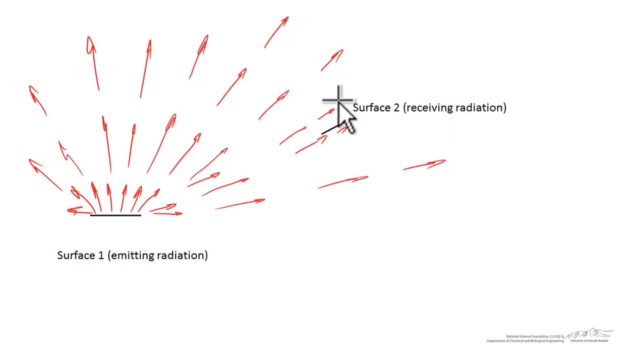 is infinitely thin, So all the radiation just scoots by in both directions and it's not receiving any radiation in that case. So that's one example or one thing to consider. Another thing to consider is the location of surface two relative to surface one. So if I put surface 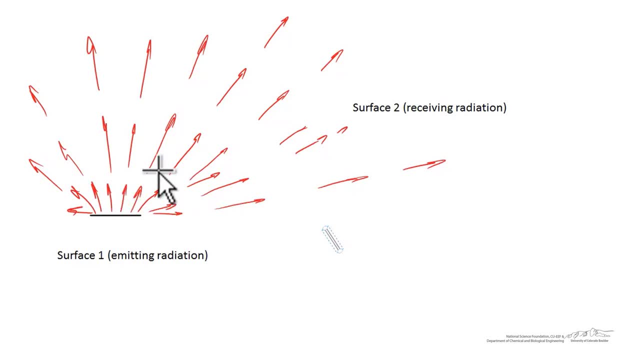 two down here, it's pretty obvious that it's not receiving any radiation in that case. So if I do, if I even drew horizontal arrows, radiation coming from one it's going to be for this. It's below even those arrows, And if I bring it up, the amount of radiation 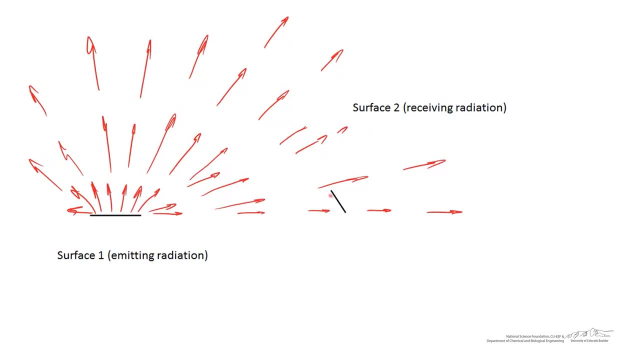 received here the surface area, that surface two. the surface area that surface two sees of surface one is really small if I position it here. Conversely, if I take this and I put it right over the heart of it, or if I move it up into this field, up in here, the surface. 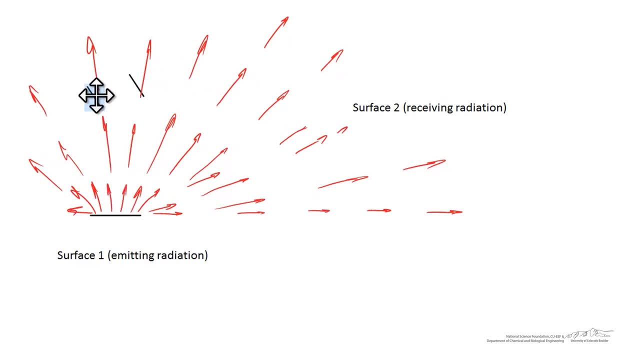 area that it sees. the projected surface area is much bigger if it was located up in this region, for instance. So in this case this would be the maximum amount of radiation that surface two could feel. It's arranged perpendicularly to the radiation and it's right in front of surface. 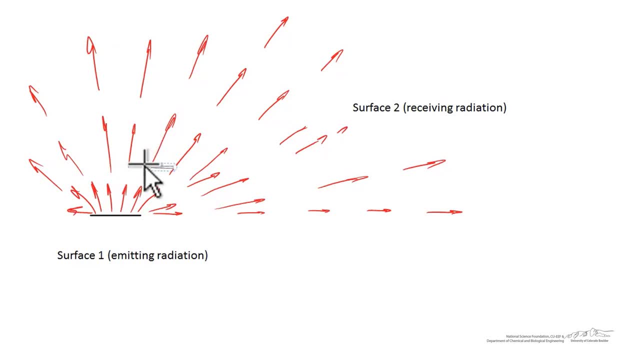 one. So it's a couple of things to consider and we'll talk about those mathematically in a second. So I've gotten rid of that. all the radiation field and I'm going to draw one ray coming from surface one to surface two And we're going to say these are differential elements. 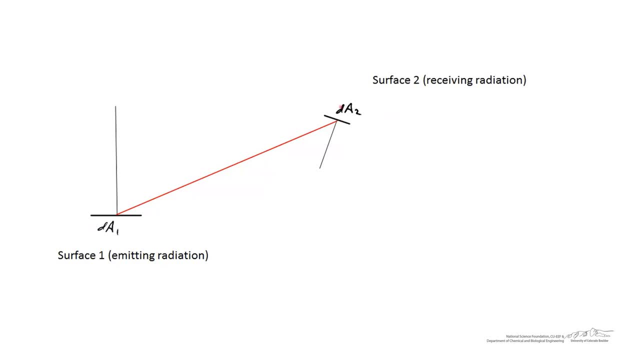 so they're really small surface area And I'll call them dA1 and dA2, because they're dA2- to emphasize that this is really only a good approximation if they're both small. We'll get into some more complicated stuff later. 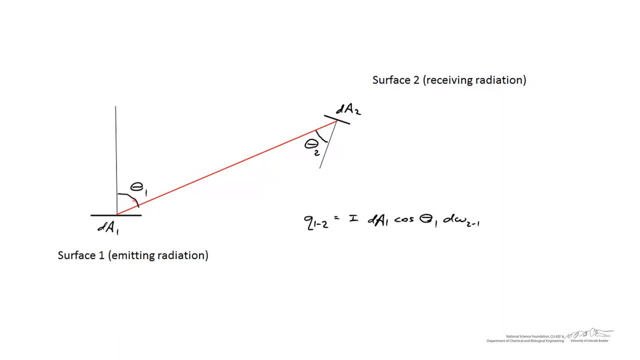 So I've drawn a single ray and I've drawn two angles: theta one, which is the angle from the normal for A1, and theta two, which is the corresponding angle from the normal to A2.. Let's say, we want to figure out the rate at which A2 is intercepting radiation from surface. 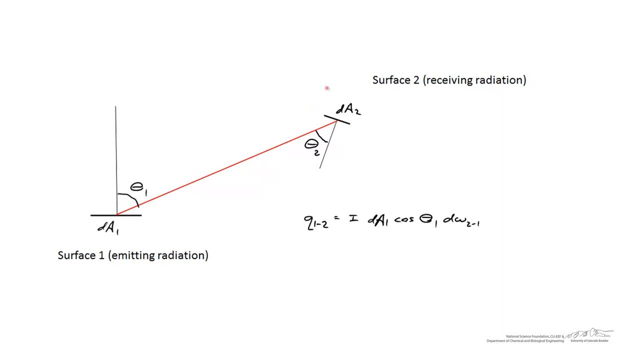 one. So we want to figure out the rate in total watts that A2 is receiving radiation. So this is the working equation that we can use in this situation. I'll explain what these terms mean. So here we've got Q12 is the rate of irradiation that's intercepted by A2 that was generated. 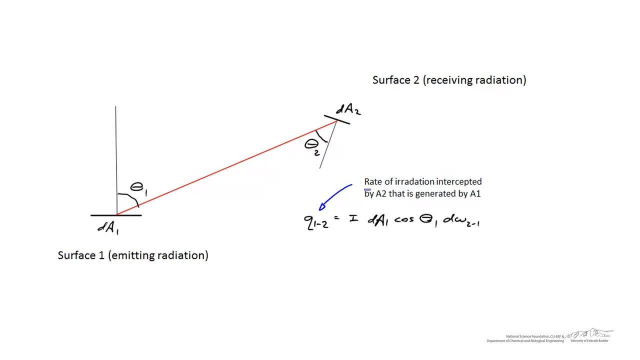 by A1. So we want to figure this out. And the units on this, we want to figure them out in watts, so the total wattage of radiation intercepted by A2.. This parameter I is called the intensity of radiation that's emitted by surface: A1. So 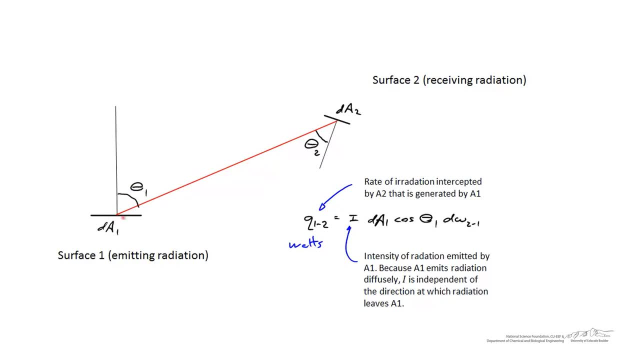 it's because A1 is emitting radiation diffusely. I doesn't depend on the angle, it doesn't depend on this angle, theta one. So we can say I coming off in this direction, or this direction, or this direction, this direction. I would be the same in all of these cases. 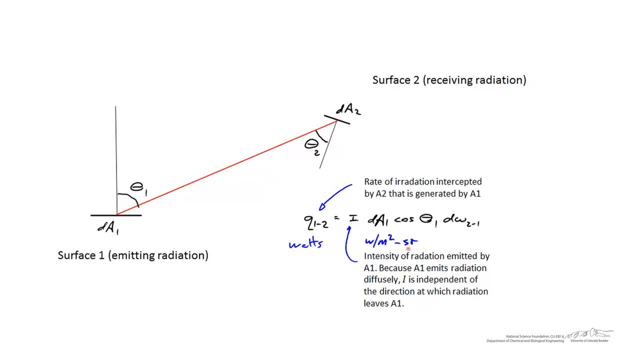 The units of I are in watts per meter squared per steradian, So it means the wattage emitted by surface. one per square meter of surface, one per steradian. So SR is watts per meter squared per steradian, abbreviated, an abbreviation for steradian. Now I'll talk about it in a second, but really 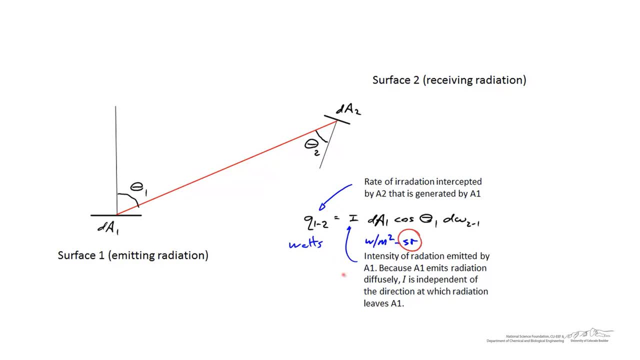 what it means is per unit area of target, almost So it's effectively how big a steradian is, effectively, how big is your target, or how big is the target? in this case, the target is A2, how big does that target look compared to A1. This term, dA1- cosine theta1- is simply 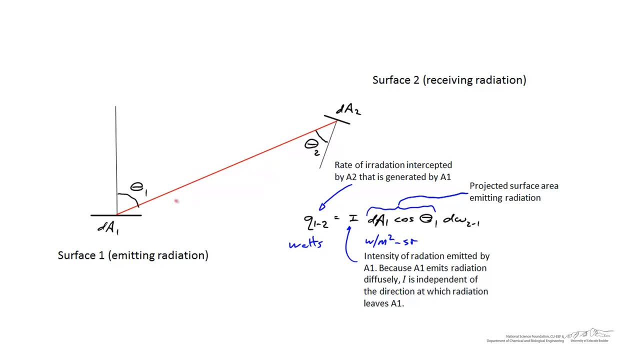 the projected area, the projected surface area emitting radiation. So we talked about it in the beginning. if theta1 was, let's say theta1 was- 90 degrees, that would mean that this differential area would be lined up like this and there would be no projected 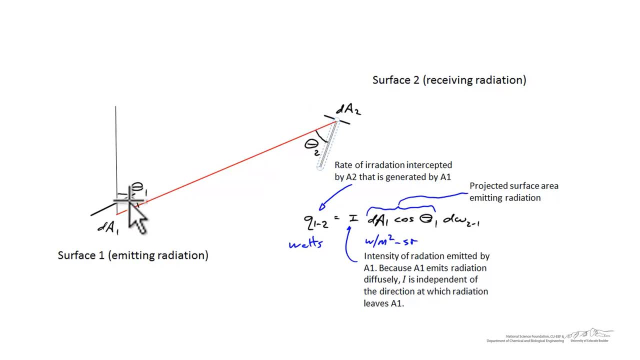 surface area for dA2 to feel So it would be. effectively, it wouldn't be shined down at all because this surface is infinitely thin- if theta1 was in that direction. But as it is, theta1 in this case looks like it will be about we could estimate theta1's 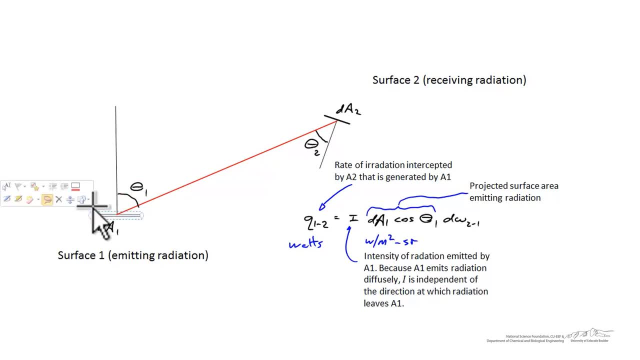 60 or 70 degrees, something like that. And if we took theta1 and theta2 and theta3 and theta4 and theta5 and theta6 and theta7 and theta8 and theta9 and theta10 and theta11 and we tilted it 90 degrees to the array, 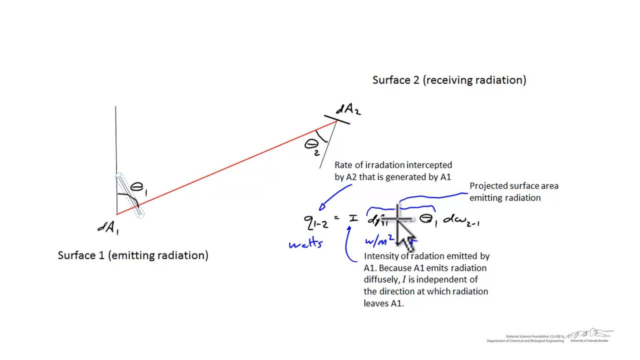 theta1 would be equal to 0, we'd have to cosine: theta1 of 0 would equal 1 and the projected surface area would simply be this surface area. And finally, we've got this d omega21, and it's defined as the solid angle subtended by A2 when viewed by A1. So, in essence, this, 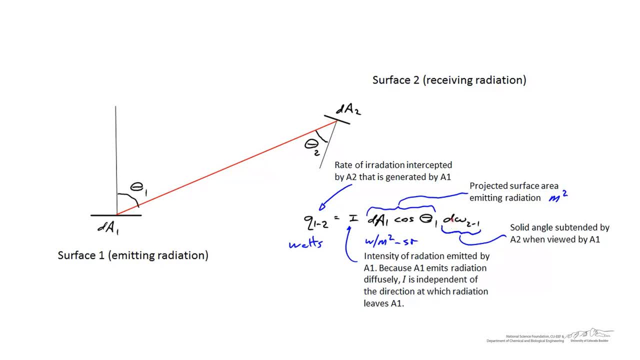 d omega is the size of the target and if we wrote it out well, the units on d omega21 are in steradians. If we write it out mathematically, d omega21 is the surface area of the normal projected surface area of A2 divided by R squared. So R is the distance between the. 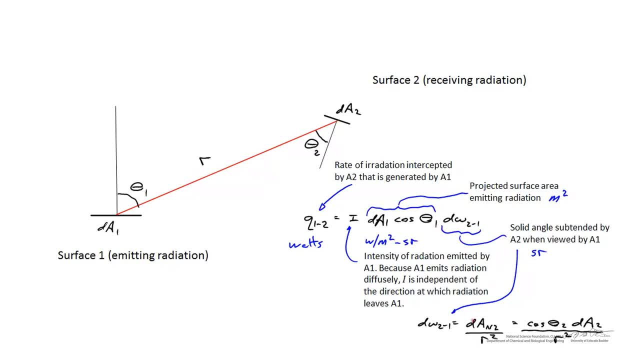 center of dA1 and the center of dA2.. And this is the projected surface area of A2, so we just say cosine of theta2 times the differential area of A2 divided by R squared. So you could look at this a couple of different ways. We could say: if you imagined, if you've ever been, 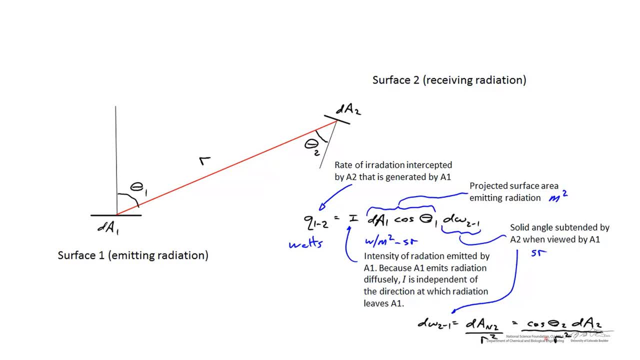 target shooting and you look at a target. if the target was only 5 feet in front of you, it looks like this huge thing and there's no way you'd miss it with your rifle or bow and arrow or whatever. But at that target if you moved it back 100 yards or a couple. 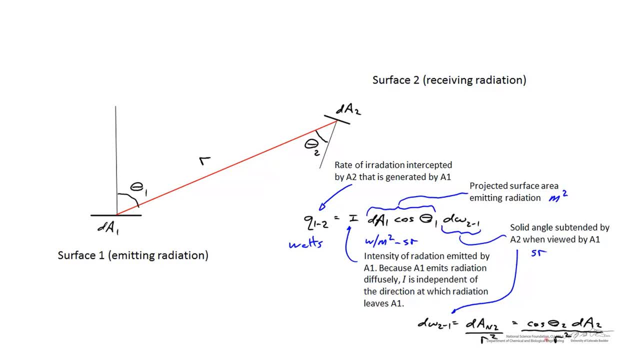 of hundred yards R? squared starts to get bigger and bigger and that target starts to look awfully small, And in this case the target dA2 starts to appear smaller and smaller when compared from dA1.. On the other hand, we could look at the surface area itself, and this is 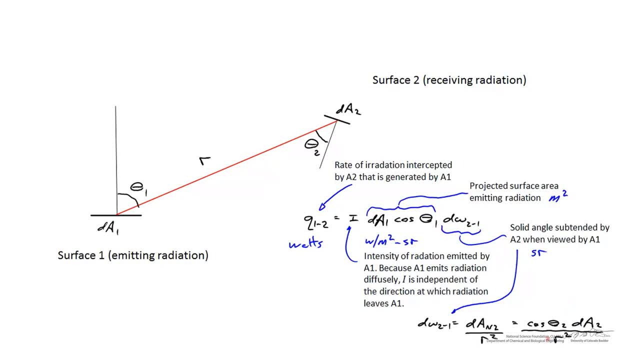 more intuitive, but you have two targets right next to one another. If R is the same, the larger surface area will appear bigger than the smaller surface area, And one other thing we could adjust would be this angle. So you might look at it this way, If this is you. 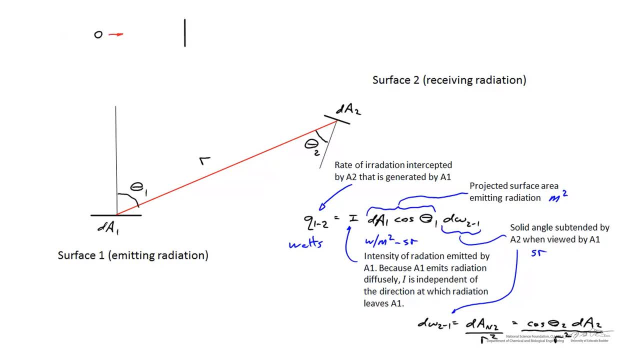 trying to hit a target. here's the target, off to the right. If I change the angle of the target- and I made it look more like this- it starts to become a real difficult target to hit. The projected area that you're looking at is the target that you're looking at. If 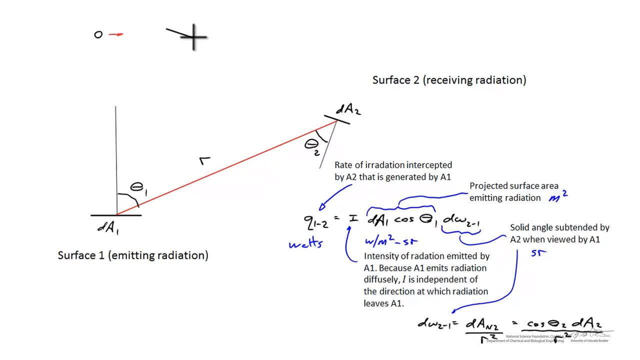 you're looking at, it becomes really, really small And in the limit. if I said, theta is equal to 90 degrees, so if I oriented the target like this, you wouldn't be able to hit it, because it's infinitely thin. It's simply a plate, And we could do the same thing. 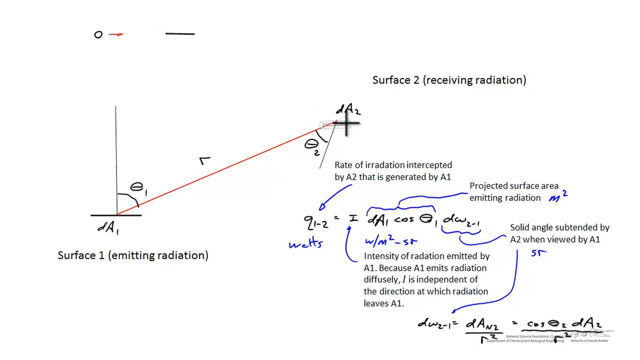 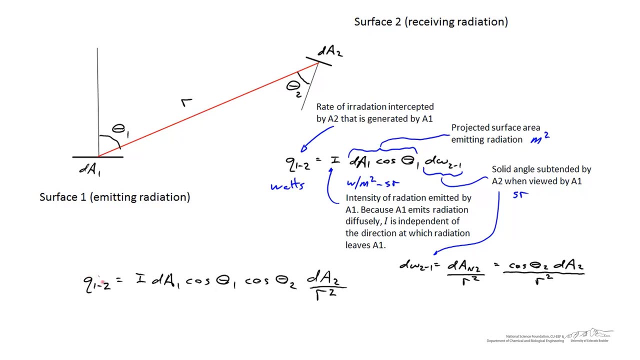 with A2.. A2, in this case, is the target, And if I made theta to 90 degrees, the radiation from A1 wouldn't be able to hit that target whatsoever. So, finally, if I put all these together, I come up with an expression for the rate of radiation, leaving one that's being 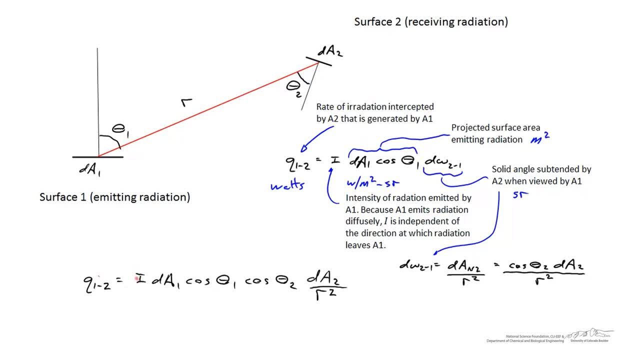 intercepted by two And it's proportional to the intensity of radiation. It's proportional to both the area of surface one and the area of surface two. Make either one of those bigger and more power would be received by A2.. And it's also dependent on the angles cosine. 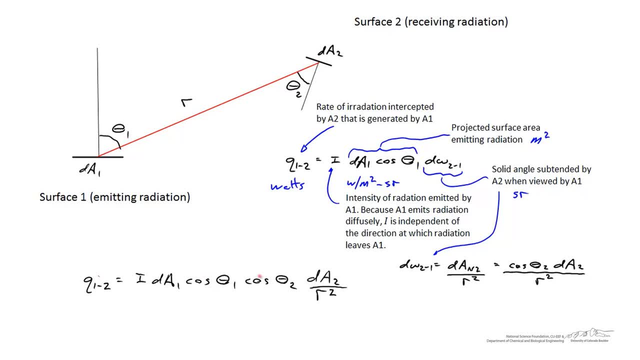 theta one, cosine theta two. like I said before, If either one of these equaled 90 degrees and there would be no radiative transfer because they would, there would be no radiative transfer because they would be 90 degrees. One surface would essentially be parallel to the radiation And finally it's inversely. 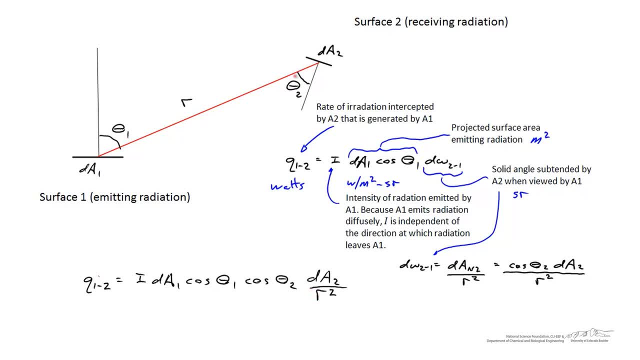 proportional to the square of the radius. So we made R really large. If we moved dA2 way far away from A1, we put it way out in here, it would receive a lot less radiation from A1 than, say, if we moved it, if we moved it real close. So I took A2, if we put it. 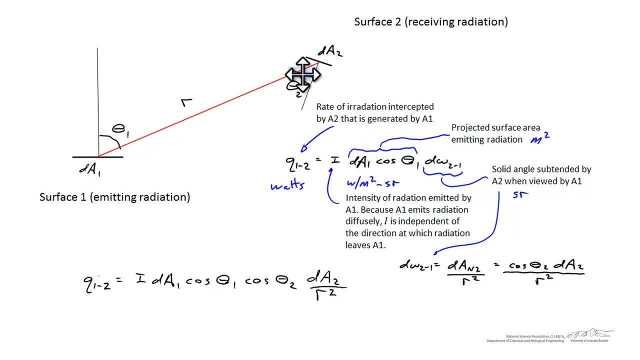 up in this region, you can imagine it receives a lot more radiation than if it was moved way back in here. So one last thing to do with the terminology. this rate of radiation I said was in watts And you'll also see irradiation by itself. So instead of seeing the rate of irradiation, 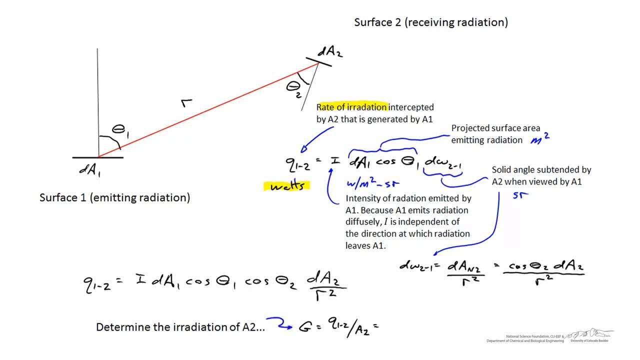 if the question asks you to determine the irradiation of A2, it means to determine G, which is Q12, so the total wattage divided by the surface area of area two, So Q12 divided by A2.. So you'd simply divide both sides by dA2 in this case, and we'll come up, come up.